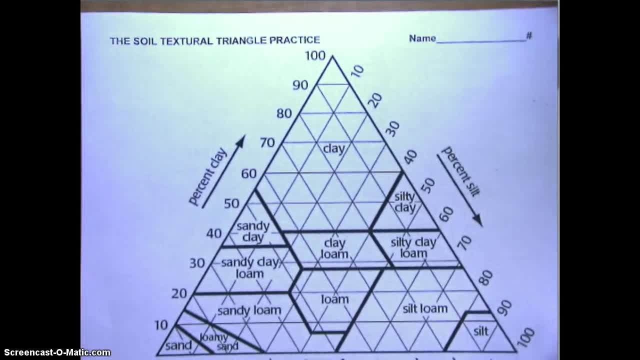 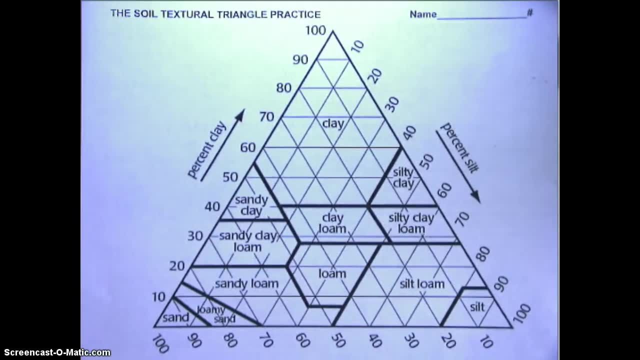 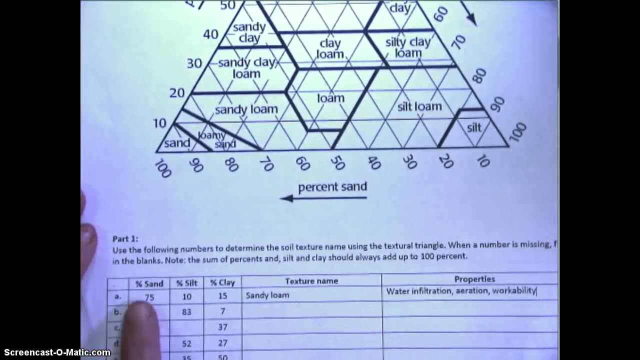 So in this video we're going to learn how to use a soil texture diagram, or it's called a soil triangle, to determine the amount of sand, silt and clay in a soil sample. So at the bottom of this sheet we have a table. The table has the 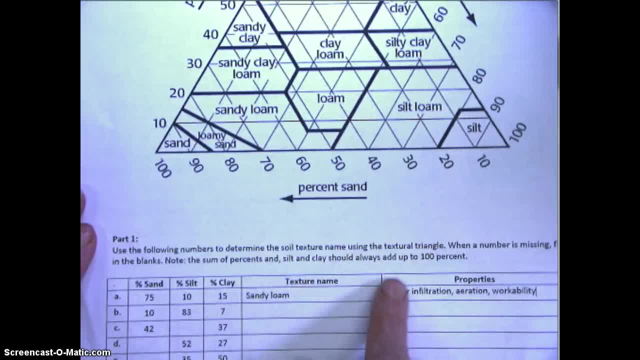 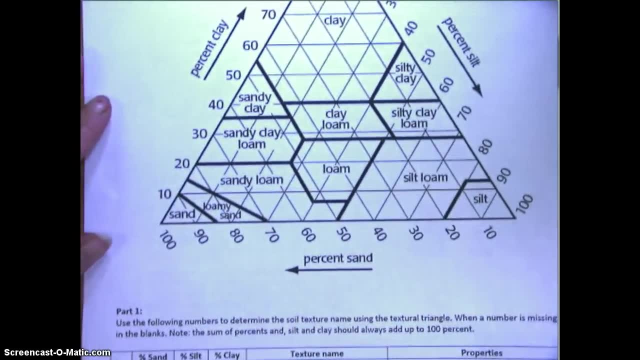 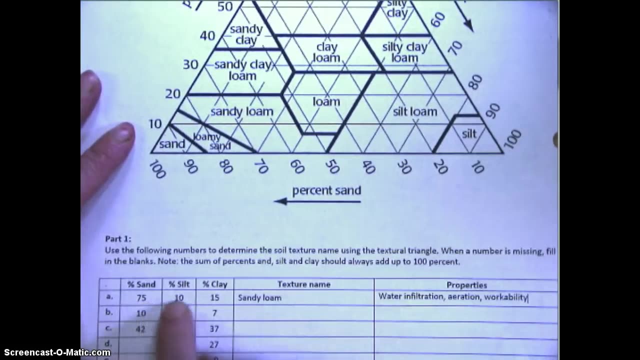 percent of each sand, silt and clay, the texture name and then the properties of that clay, which are dependent on the different types of minerals that it has. So for the first example, we have 75 percent sand, 10 percent silt and 15. 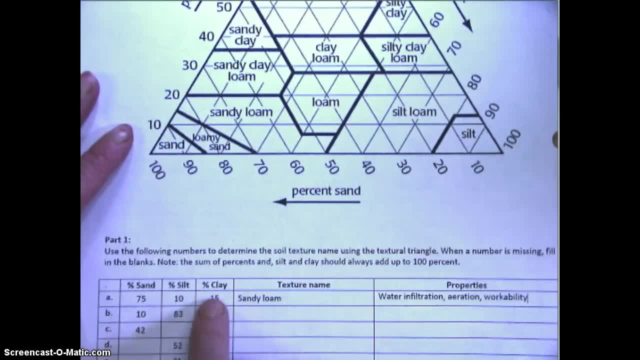 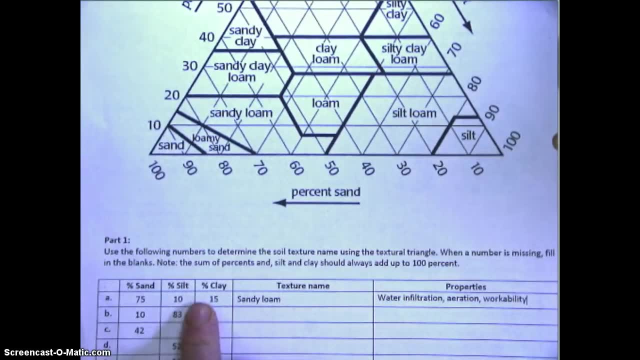 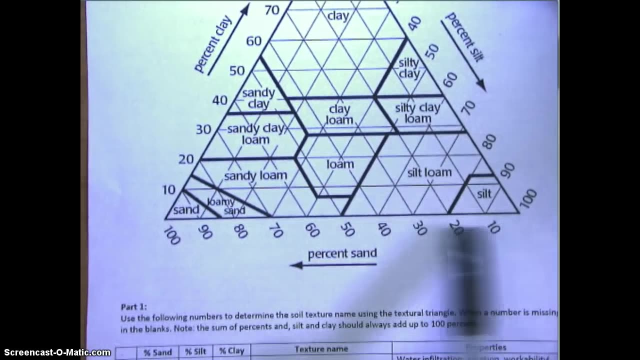 percent clay. Now remember, if you add sand, silt and clay, it makes loam. So it makes sense that that would be sandy loam. But you can figure this out by going: here's the percent sand. so there's 75 percent of that. So here's 100 percent. 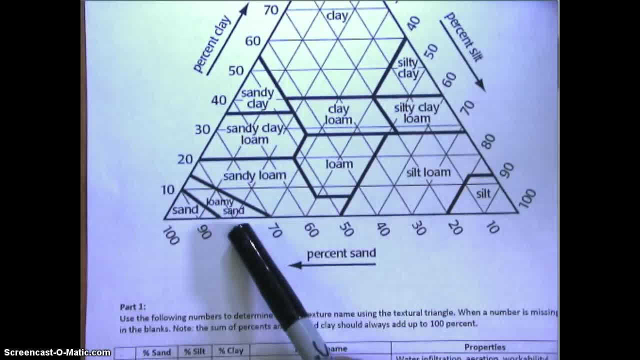 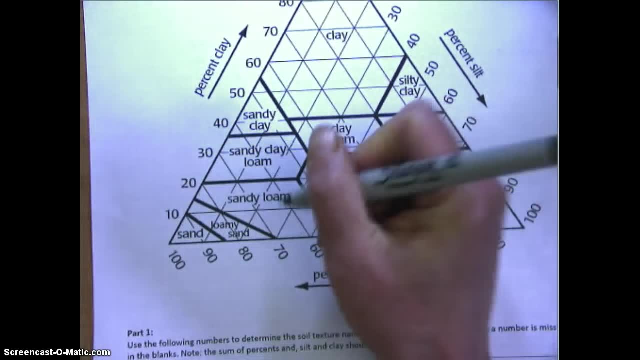 here's 70, here's 80. And there are two lines: there's one that goes on the left and there's one that goes on the right. So you're going to figure out 75, you're going to go in between 70 and 80 and 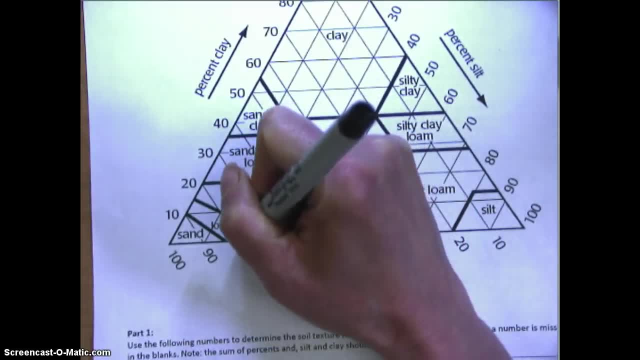 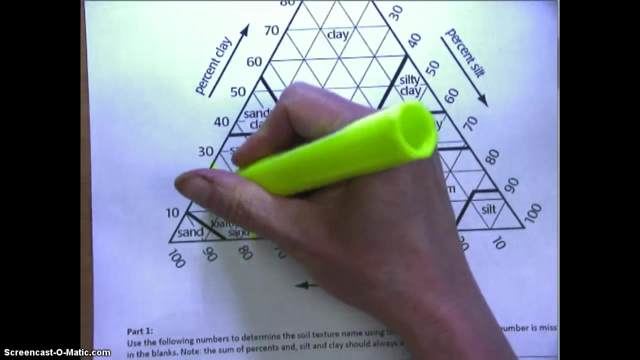 you're going to go towards the left, So in between 70 and 80 is about right here And you will just put a little. you can use a highlighter if you'd like. You're going to get in between the lines that are 70 and 80, 70 and 80. 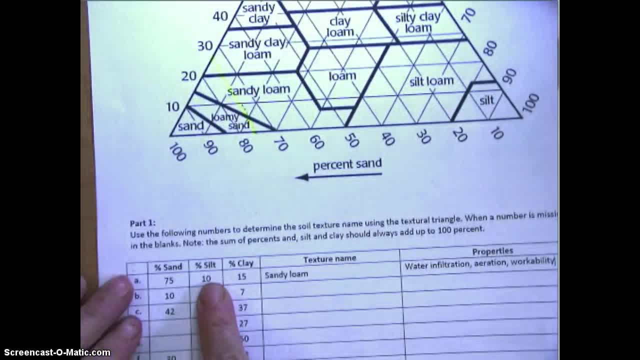 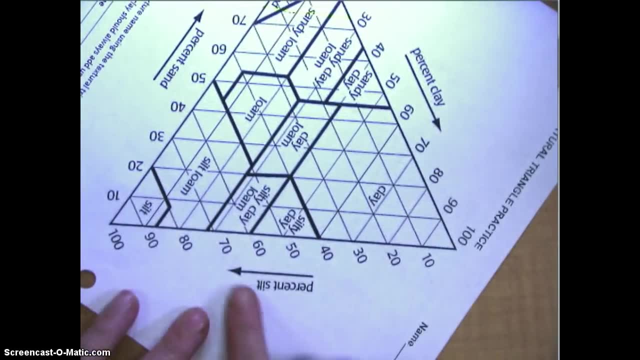 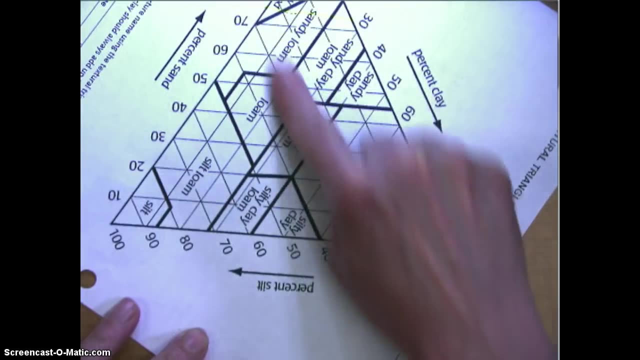 Then you're going to go figure out where's 10 percent silt. So you'll find the silt line. move the paper. So now you see that's 10 percent silt. So anywhere along this line is 10 percent, 20 percent, 30 percent. So you're always going to look. 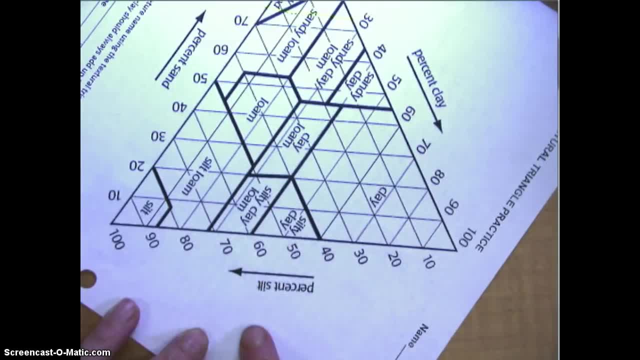 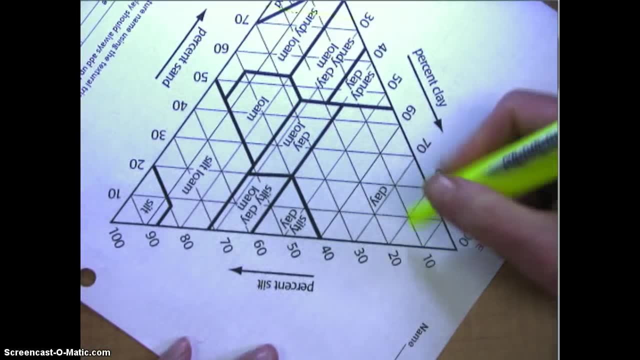 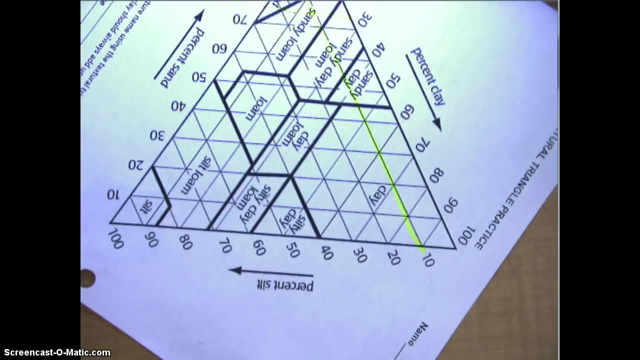 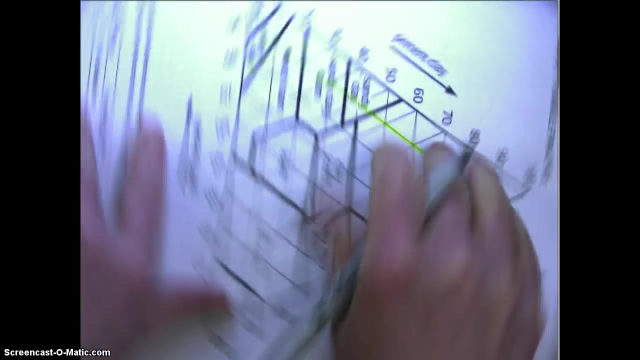 at the line on the left. Okay, so we're looking for 10 percent silt. So we'll take our highlighter and we're going to highlight 10 percent silt, And where these two lines intersect, that is should be where your clay is. So if we go to clay you want to 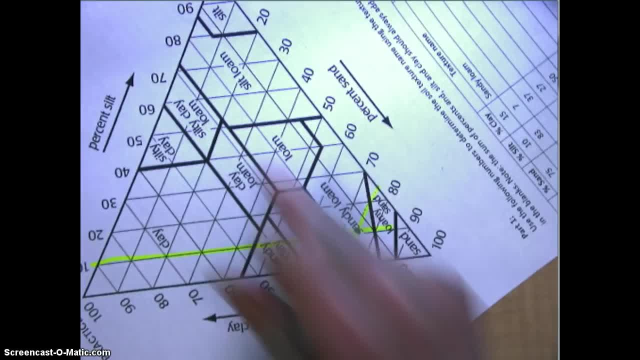 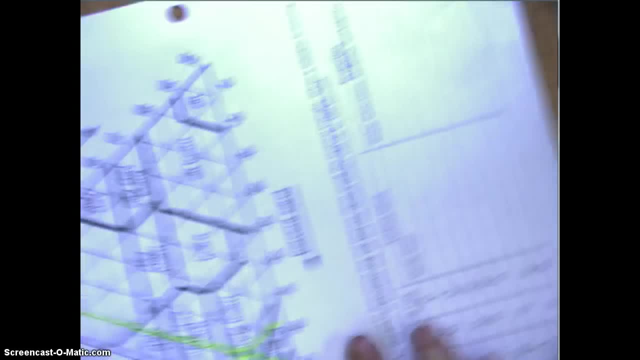 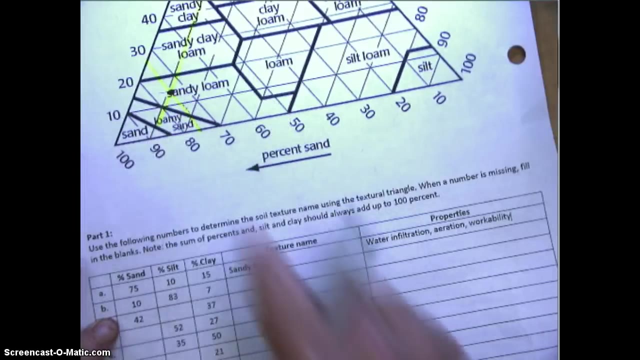 turn it to the clay side. All of this is 10 percent, 20 percent, etc. So it looks like between 10 and 20 is 15 percent. It's 15 percent clay, And indeed that was 15 percent clay. So that's where we got sandy loam here. So let's do the. 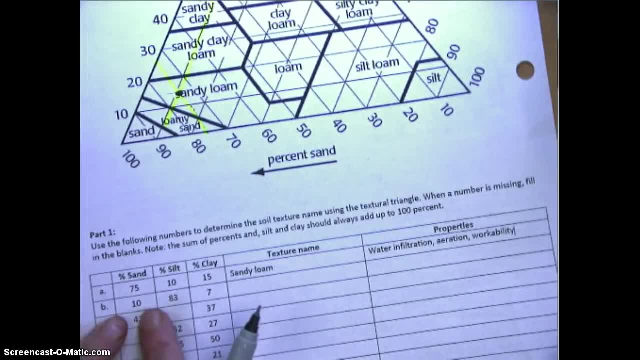 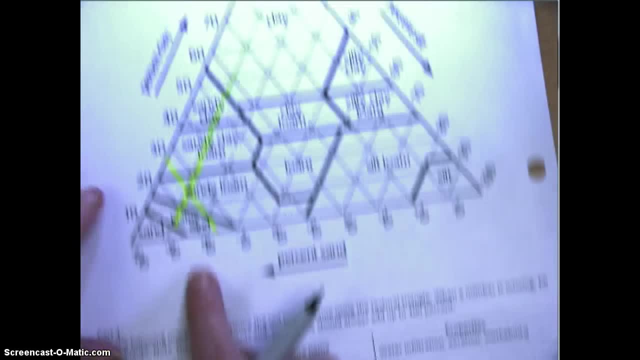 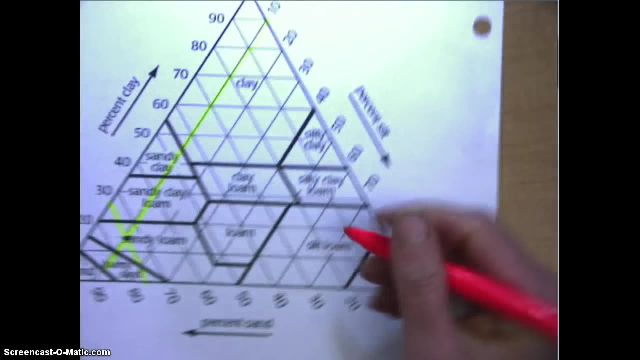 second one: together Got 10 percent sand, 83 percent silt and 7 percent clay. So we're going to go to the sand. We're going to go find 10 percent sand, So it's going to be somewhere and I might use a different color. You can start off with a. 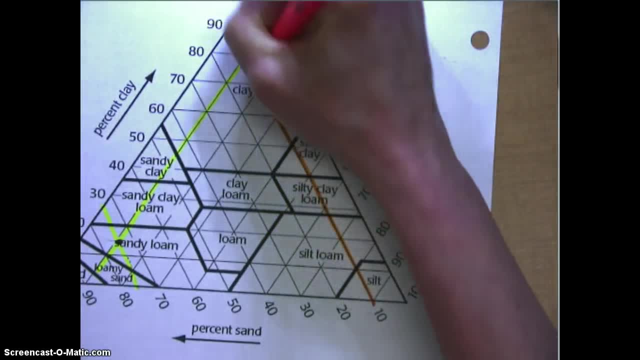 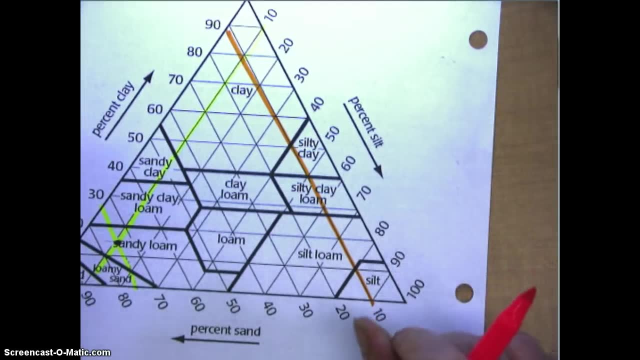 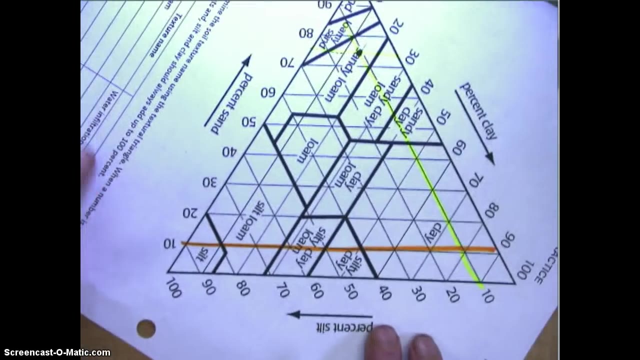 few different color highlighters. Remember I told you to go the line on the left, not the right. Now we're going to go to 83 percent silt, So you can turn it to the silt side and you will find 83.. Here's 70, here's 80, here's 90,. 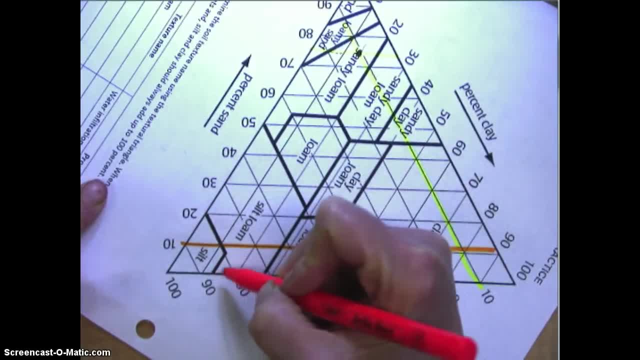 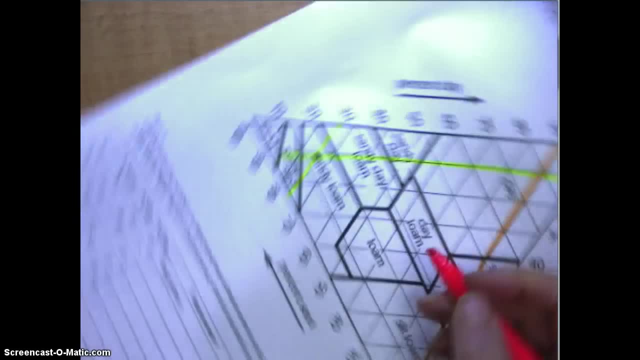 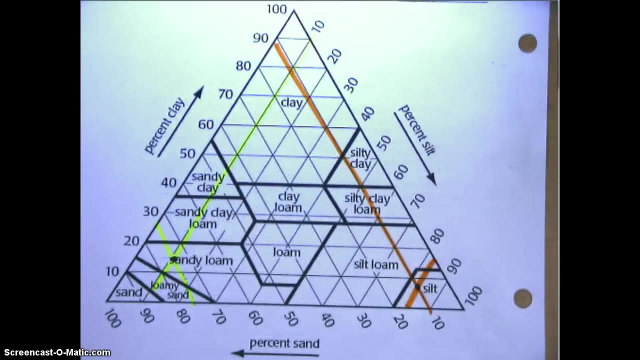 and you're going to go to the left. So 83 is probably closer a little bit closer to 80.. Okay, and so far we could figure out just based on those two that it's silt. But let's double-check: Seven percent clay. So we're going to go. 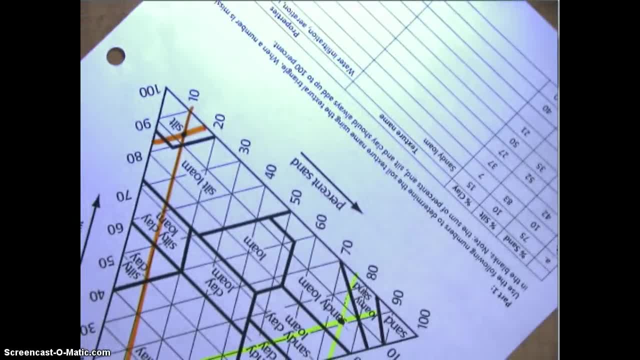 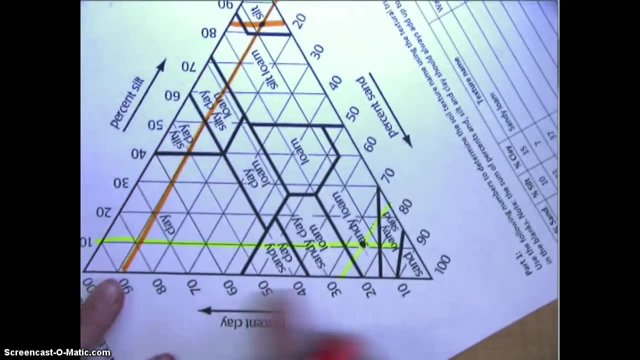 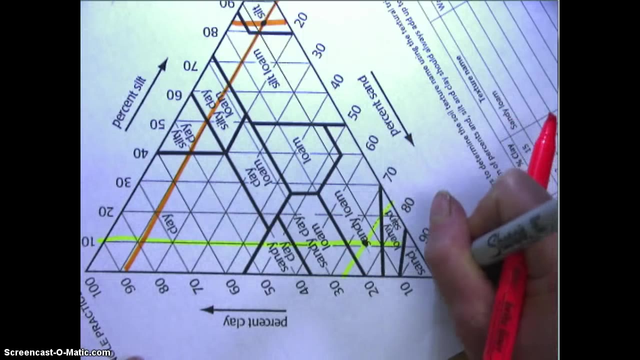 to the clay part, face it towards you, to where this line is towards you, And we're going to go to here's 10,, here's 5.. So we're going to go to 7.. So 7 would be about. 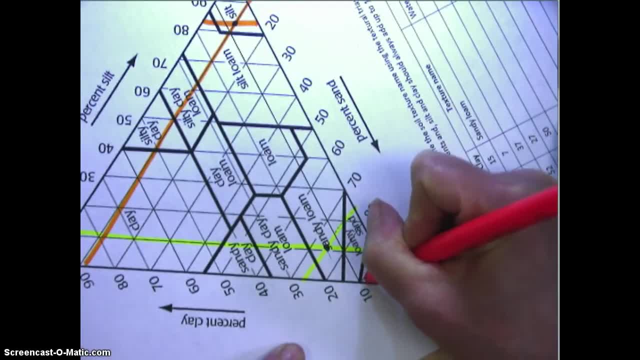 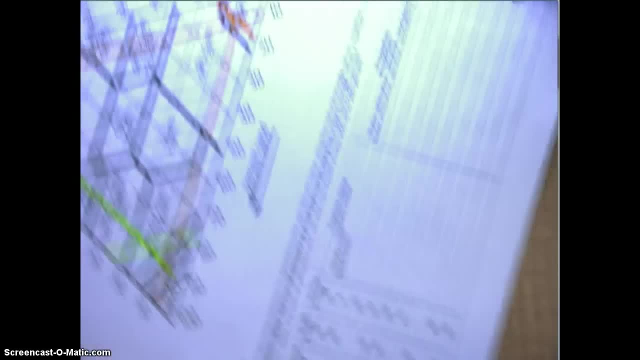 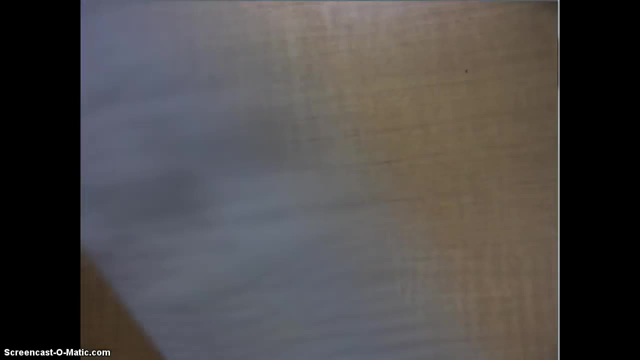 it's probably between 10 and 5.. So we're going to just kind of make a line here And indeed, boom, we're going to write silt here. Okay, so if you use the, if you look at this table here, silt has medium. 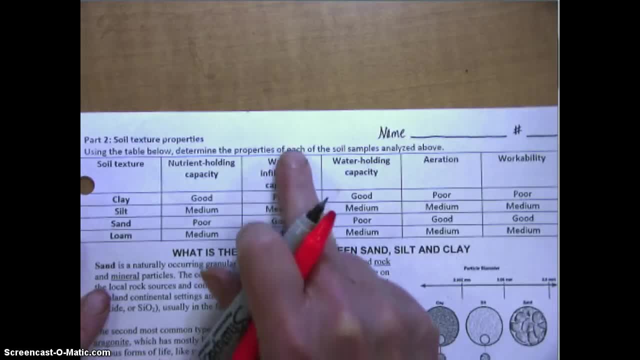 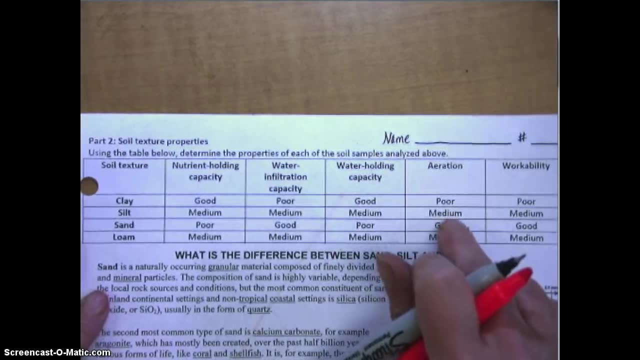 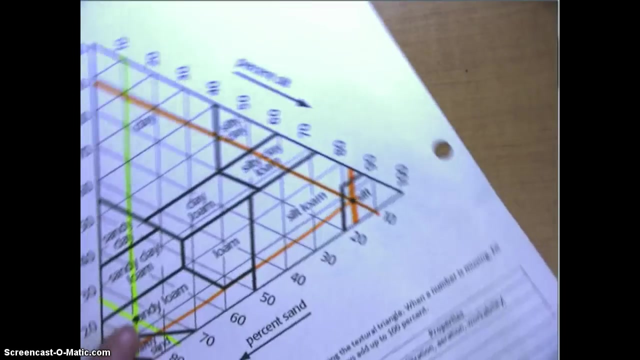 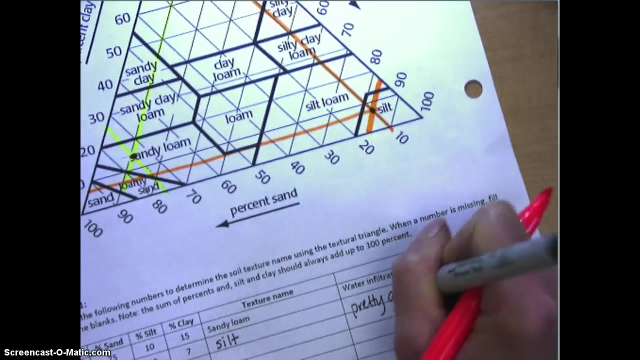 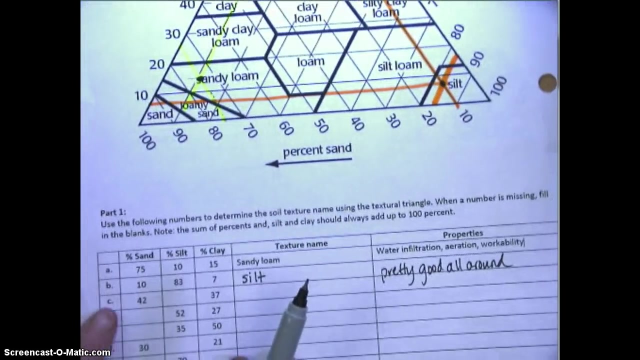 nutrient holding capacity. It filters water pretty good. It can hold water pretty well. Aeration is the amount of pore space, so it has pretty decent pore space And it's moderately easy to work with. So I would put properties under properties pretty good all around. So now let's look at this. 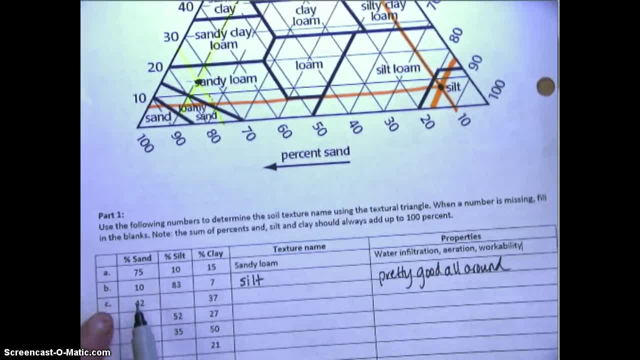 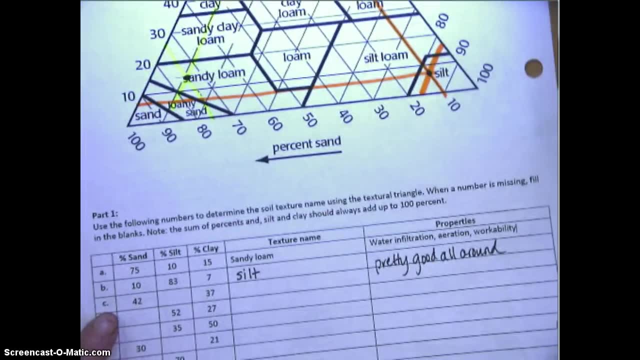 third example: C, 42 percent sand- We're not sure how much silt- 37 percent clay. So to figure out the amount of silt, the whole thing has to add up to 100.. So we'll add these two together. 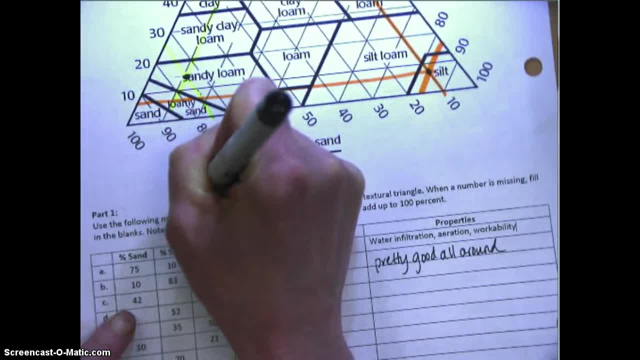 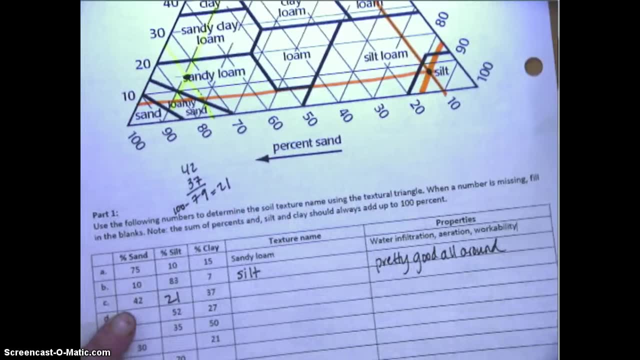 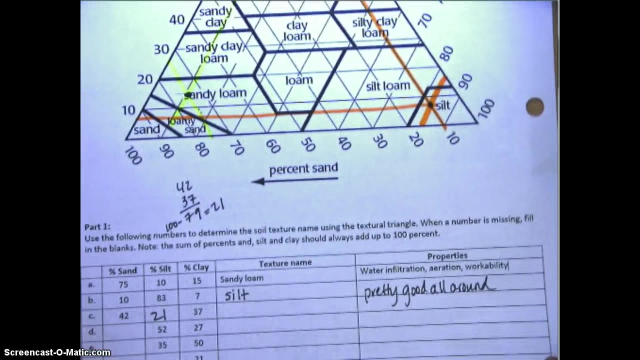 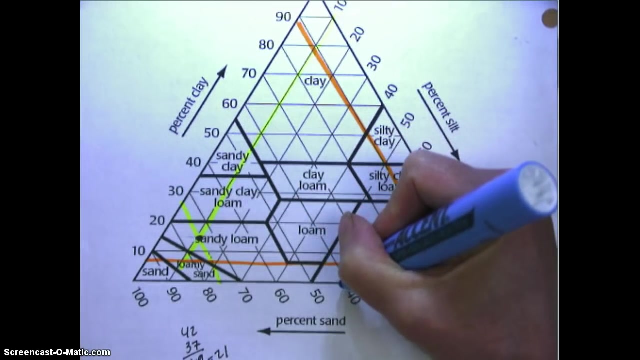 42 plus 37 is 79.. 100 percent minus 79, so that's 21 percent silt. So let's start with the sand: 42 percent sand, And I might use- I might use- a blue one this time. So here's sand: 42 percent sand. So 40,, 50, and remember: 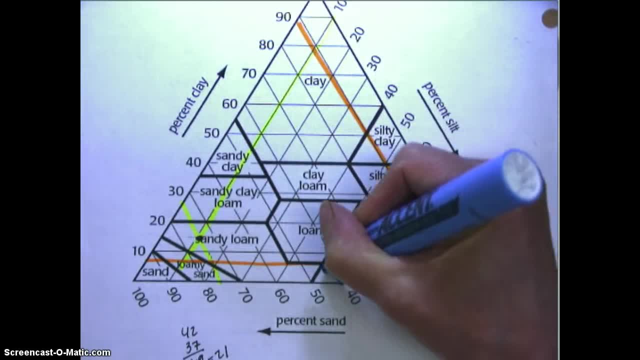 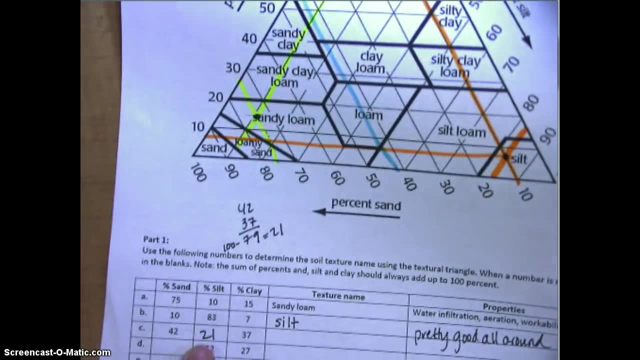 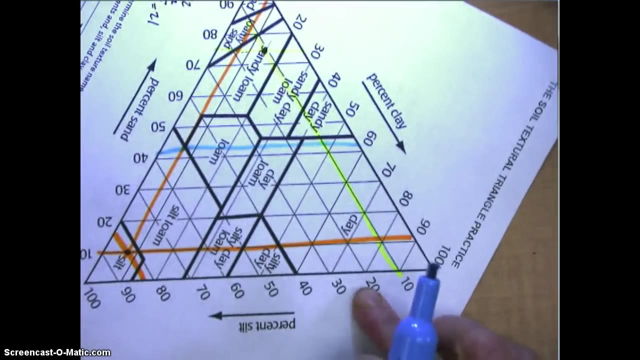 I'm always looking at the line on the left. So 42 is going to be fairly close somewhere along that line. 21 percent silt, So I'm going to go over to the silt and go to 20.. Always look at the line on the left. There's 20.. 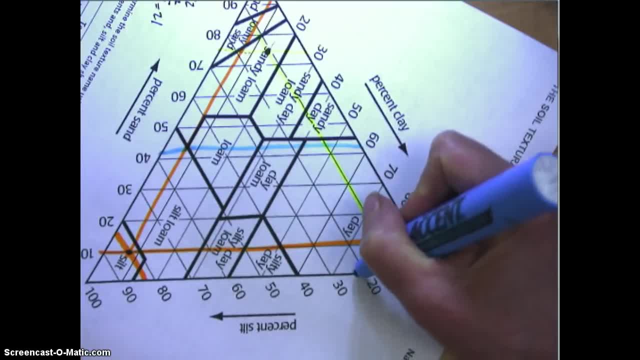 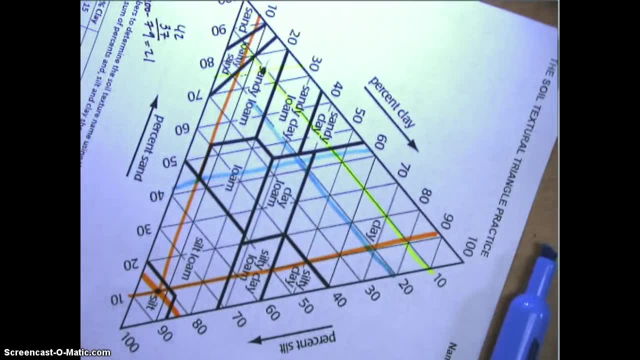 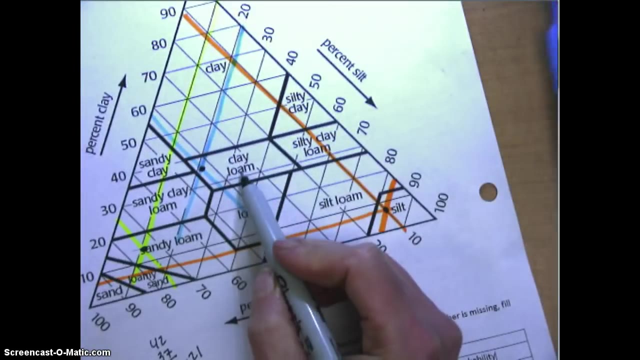 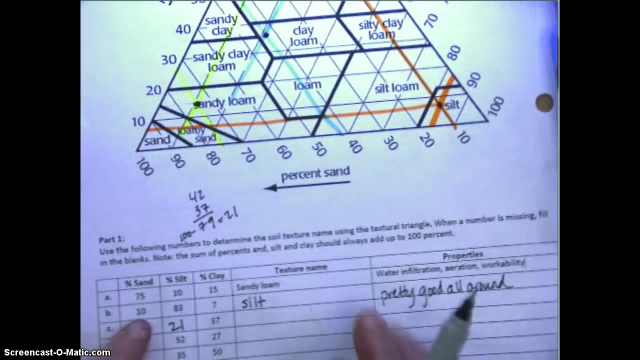 There's 30. So 21 is probably going to be close, really close to 20. And I can mark this right here And it would be classified as a clay loam. But before I totally feel comfortable with that, I'm going to double check to make sure my clay matches. 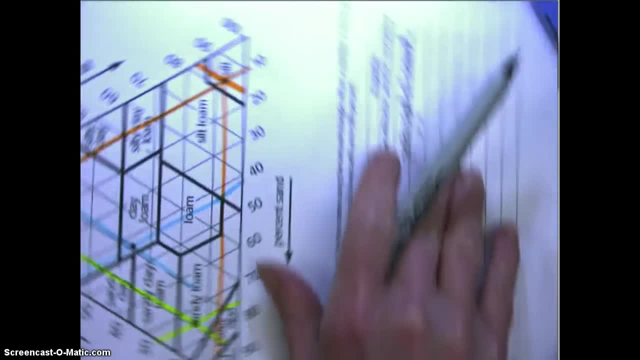 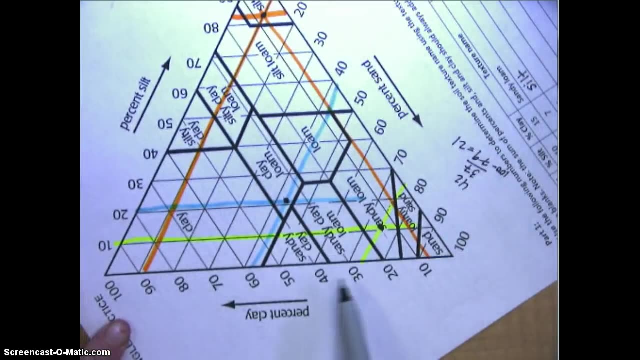 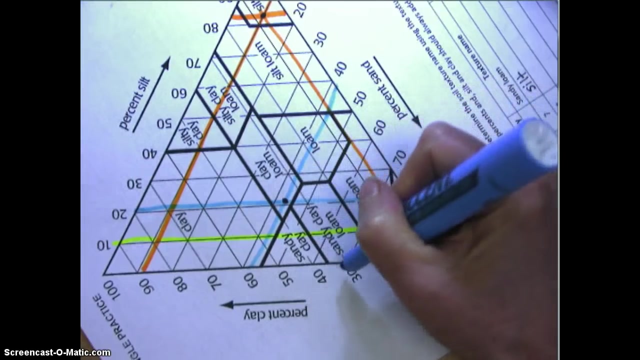 up to 37 percent. Okay, Situate it so. clay is directly in front of me, And then I'm going to find here's 30,, here's 40. And I'm looking at the lines on the left. So 35 is probably in the middle. 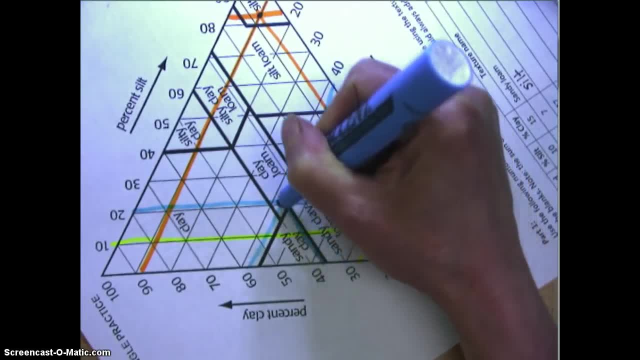 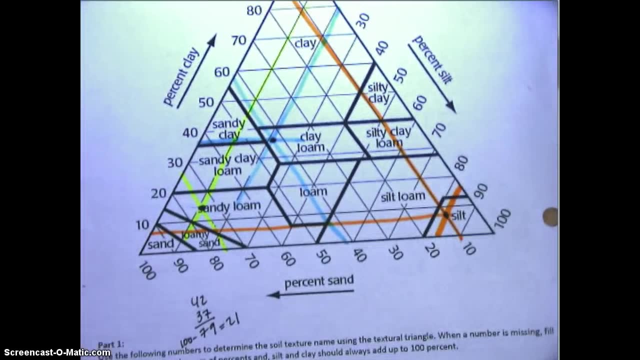 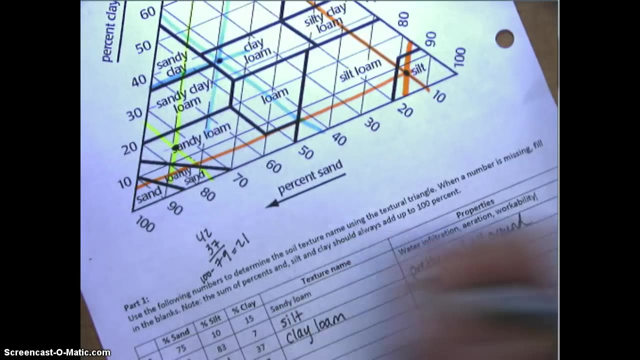 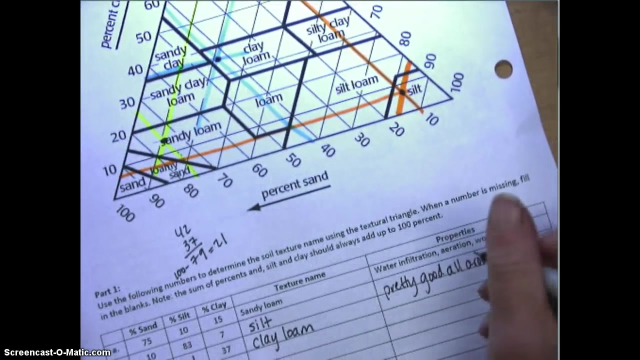 So 37 would be about right here, And so where all three of those intersect would be a clay loam, Okay, And then I'm going to go over to the silt. Okay, And clay is pretty good because it's negative in nutrients. A lot of the nutrients are positive. 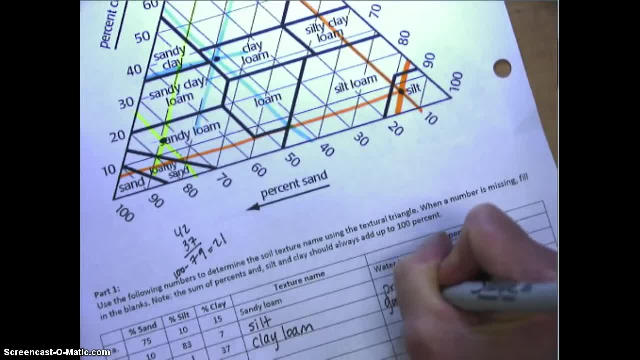 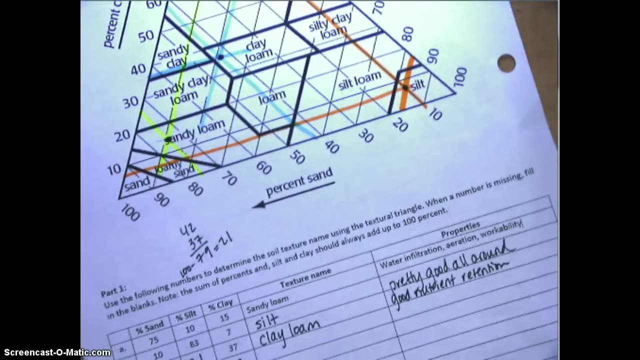 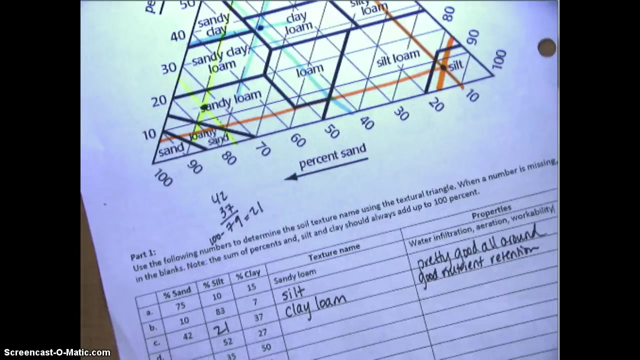 It's good nutrient retention And because it is a loam, it has good porosity and permeability is equally as good, So it's probably very workable as well, Okay, Okay. So for D, if you want to continue listening to this, then you can. I'll walk you through. 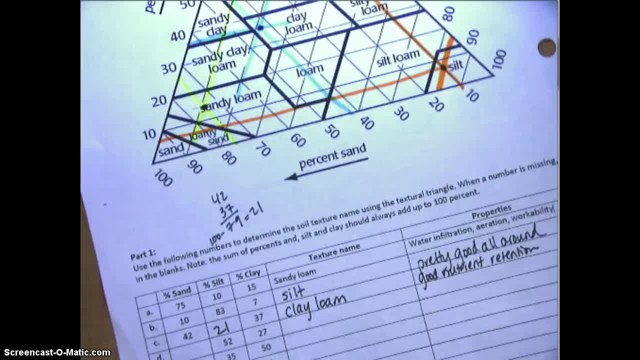 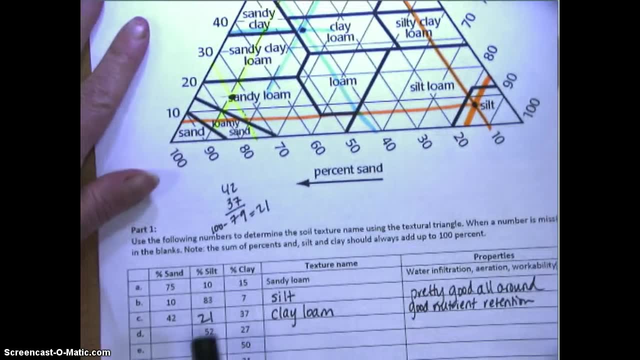 one or two more, Otherwise you can go to the end of the video and I will show you the answer key. So for D we're going to have to figure out again. 52 and 27 is 100, is 79. And 100 minus. 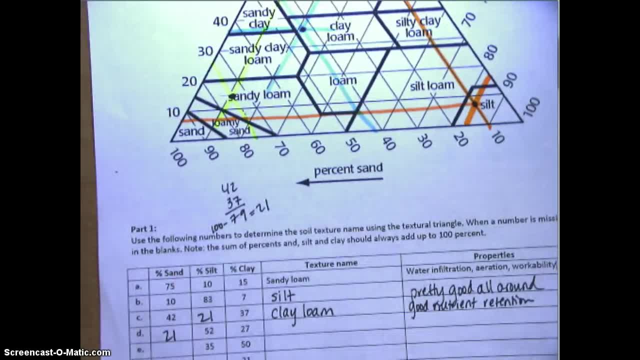 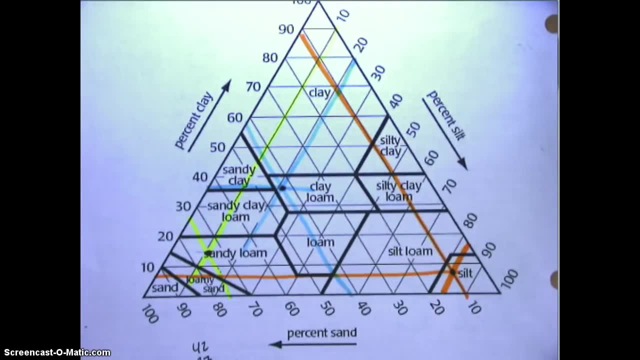 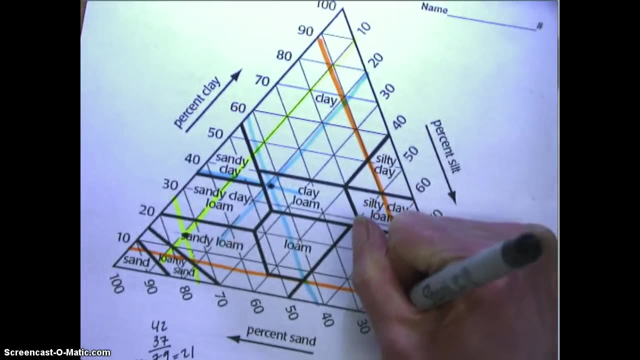 79 would be 21 percent sand. Okay, Okay, Okay. So we'll start with the chart 21,. and I'm just going to do it in this pen here. So 21 percent sand would be somewhere around in here. Remember you're going to go, not the. 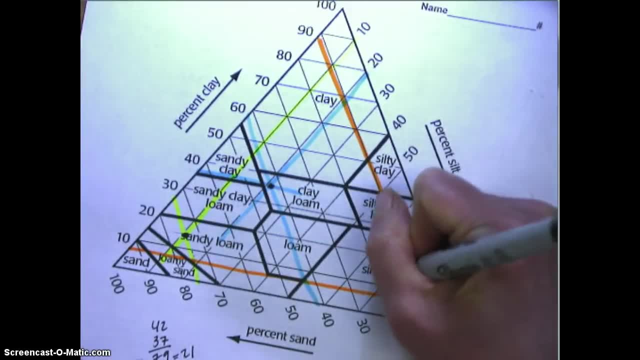 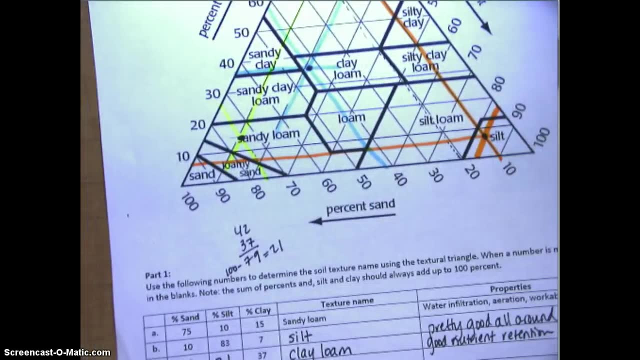 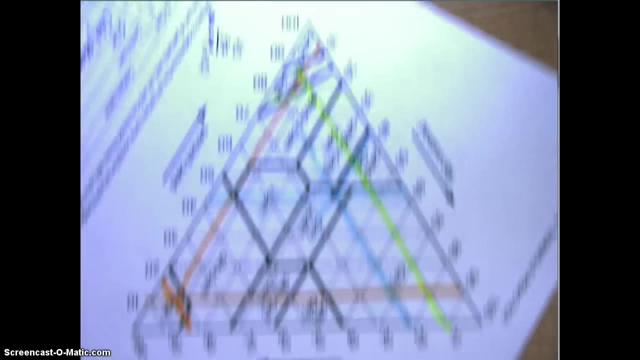 right line but the one that goes to the left. So, 21 percent sand. How much silt? 52 percent silt. So I'm going to get over to the silt. Have that right here. Okay, Okay, Get that right in front of me. Here's 50.. Here's 60. So 52 is going to be again on. 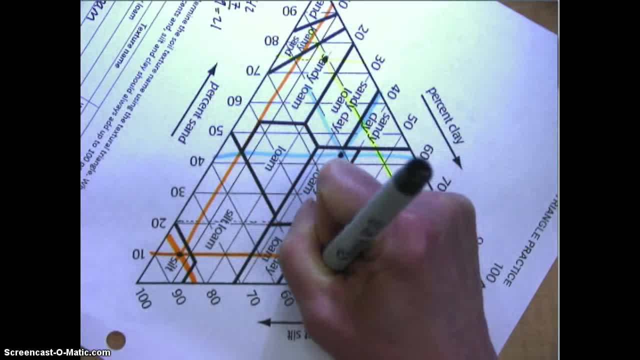 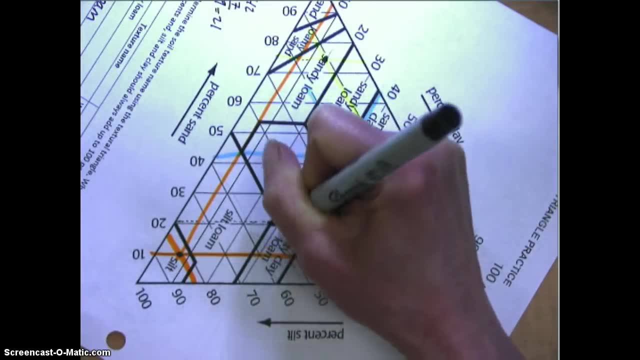 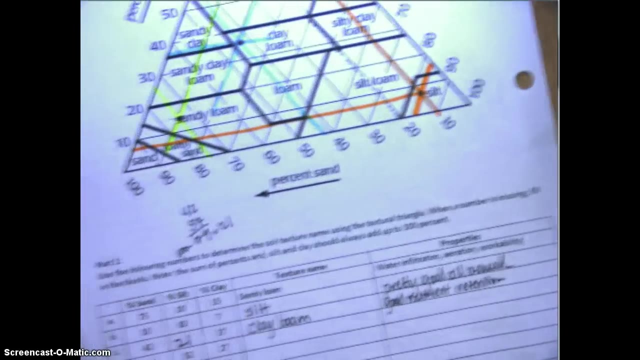 the left. It's going to be between this line and this line, So 52, it's going to be somewhere in 52, might be somewhere kind of on that line. Let's do, let's figure out how much clay there is- 27 percent clay. So I'm going to. 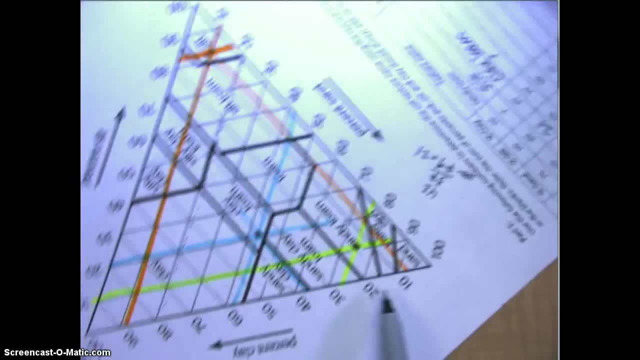 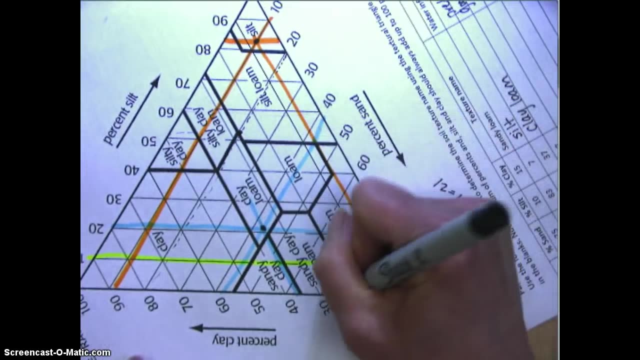 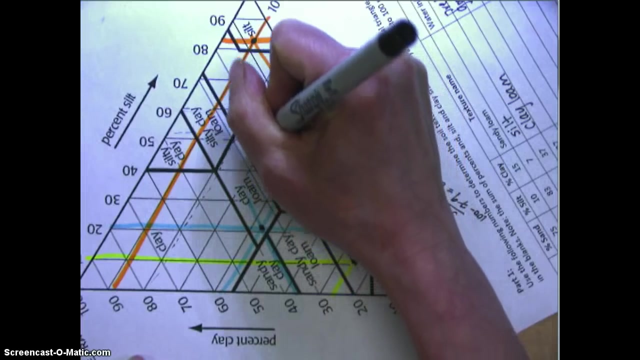 go back to the clay here. Yeah, Okay, have that right in front of me. I'm looking for 27%, so here's 20, here's 30, here's 25, so 27 would be somewhere in the middle here, and I'm gonna go all the.